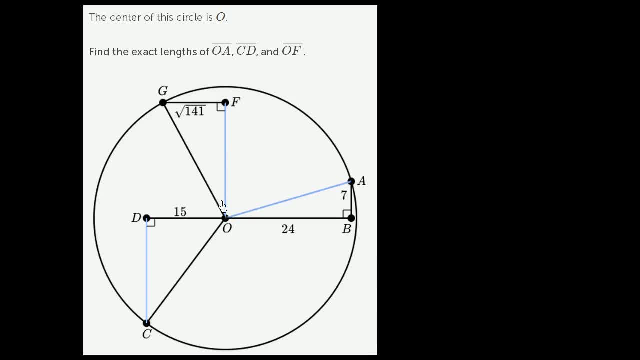 OF is one of the two shorter sides of a right triangle, But we don't know its hypotenuse either. Now let's look at OA. OA is the hypotenuse of a right triangle, And they've given us the two other sides. 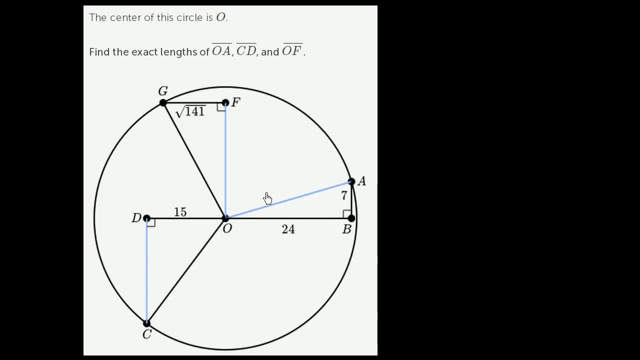 So we can use the Pythagorean theorem to figure out the hypotenuse. So we know that 7 squared- Let's call this x. We know that 7 squared, 7 squared plus 24 squared, is going to be equal to the length of OA squared. 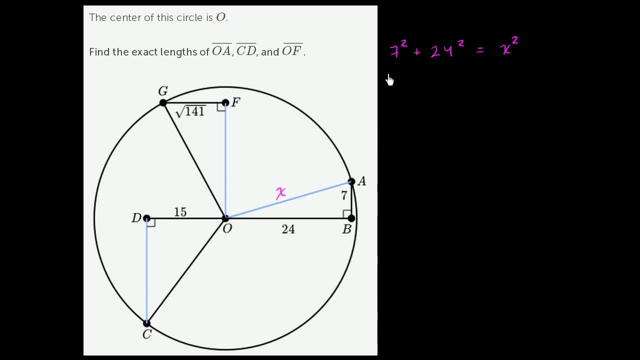 It's going to be equal to x squared 7 squared is 49.. And 24 squared? let's do a multiplication right over here to figure out 24 times 24.. 4 times 4 is 16.. 4 times 2 is 8 plus 96.. 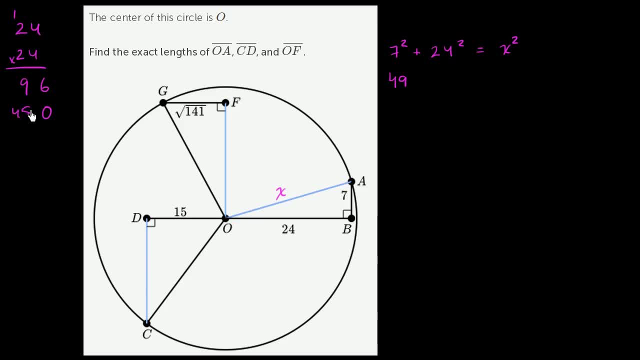 And then 2 times 24 is 48.. Add them together, We get 6.. 9 plus 8 is 17. 576.. So 49 plus 576 is equal to x squared, And so let's think about what this is going to be. 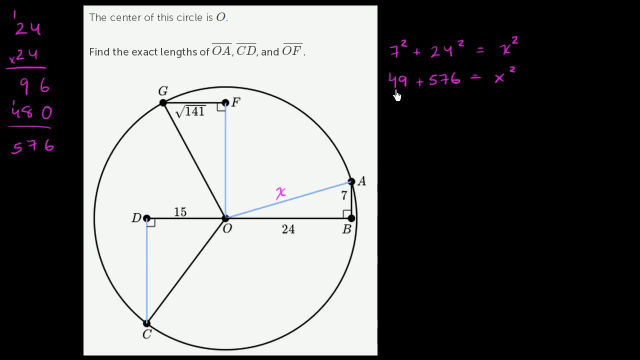 This is going to be the same thing as 50 plus 575.. I just took one away from this and added one here. So 50 plus 575 is 625. So 625.. So 625 is equal to x squared And you might recognize that 25 times 25 is 625.. 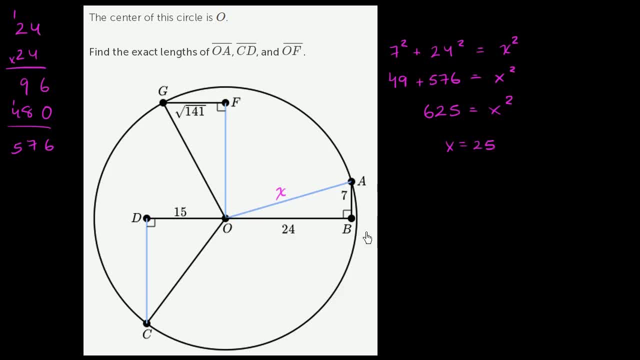 So x is equal to 25.. And if you want- don't believe me- you can multiply that out on your own. So x is equal to 25.. Or another way of thinking about it: the exact length of OA is equal to 25.. 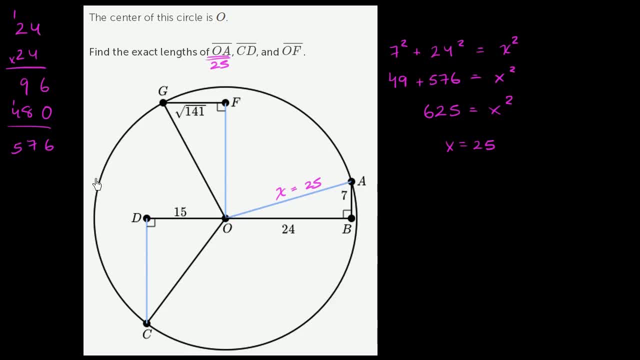 Now, how can we somehow use that information to figure out this other stuff? Well, all of these other right triangles, all of their hypotenuses, are a radius of the circle, And so is OA. OA is a radius of the circle. 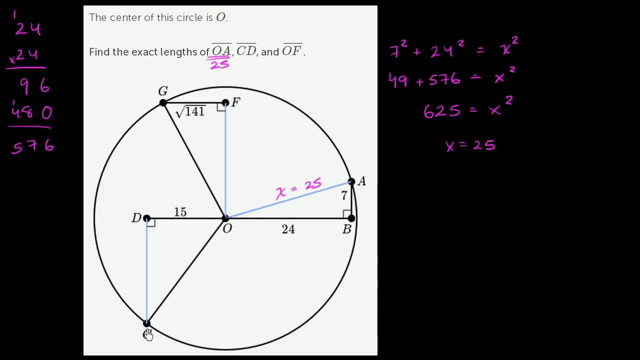 OG is a radius of the circle. OC is a radius of the circle. Well, we just figured out that the radius of the circle is 25.. So OG is going to be 25.. And OC is going to be 25 as well. 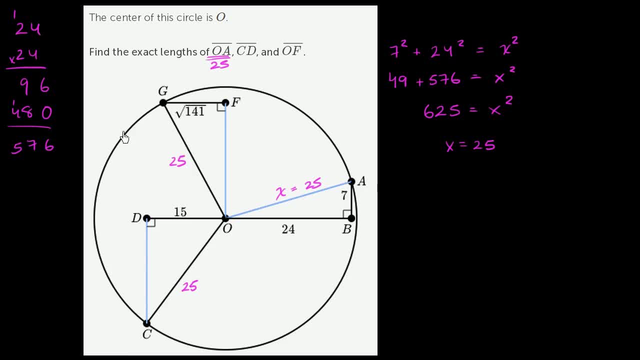 So now we just have to apply the Pythagorean theorem a few more times. So right over here, if I call OF, let's just call that. I don't know. for the sake of argument, let's call that length equal to a. 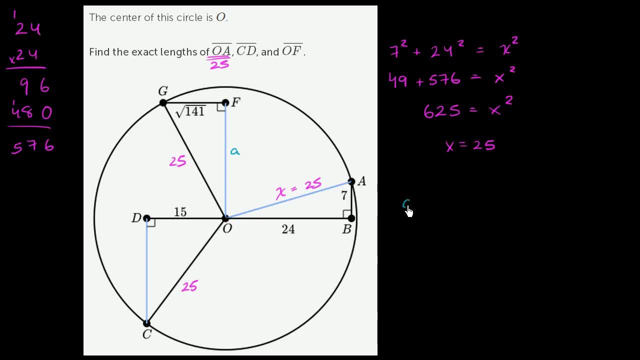 So here for this triangle we see that a squared plus the square root of 141 squared. I'll just write that as 141.. So plus 141. 141. 141. 141. 141. 141. 141.. 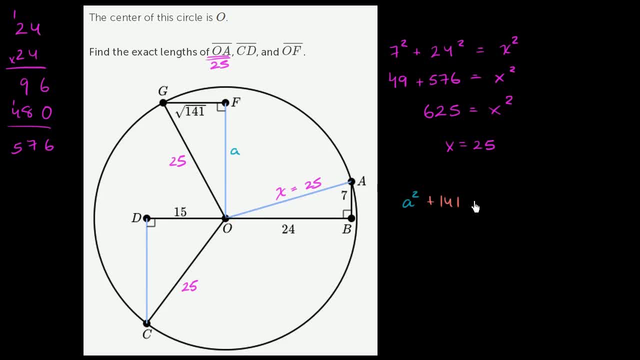 is going to be equal to 25 squared, which we already know to be 625.. It is going to be equal to 625.. If we subtract 141 from both sides, see where do we get. So let's redo: 625 minus 141, we get 5 minus 1 is 4.. 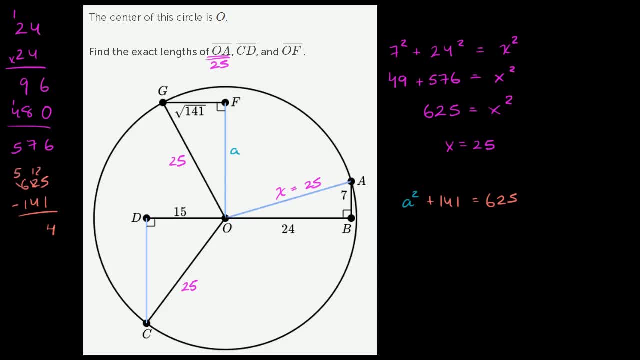 And then let's get a 12 here and then get a 5 there. 12 minus 4 is 8.. 5 minus 1 is 4.. So we get 484.. So we get a squared is equal to 484.. 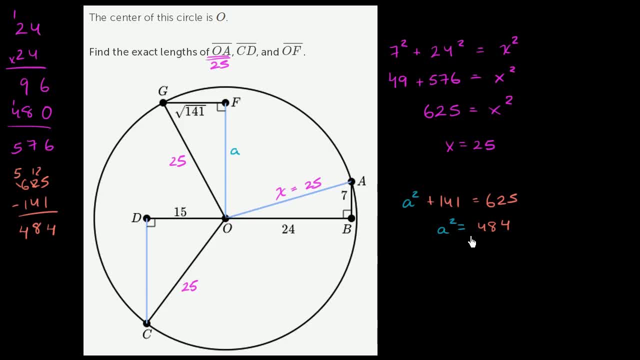 So what squared is equal to 484? Actually, I'll just try to do a prime factorization here to figure this out. 484 is 2 times 242, which is 2 times 121, which is the same thing as 11 times 11.. 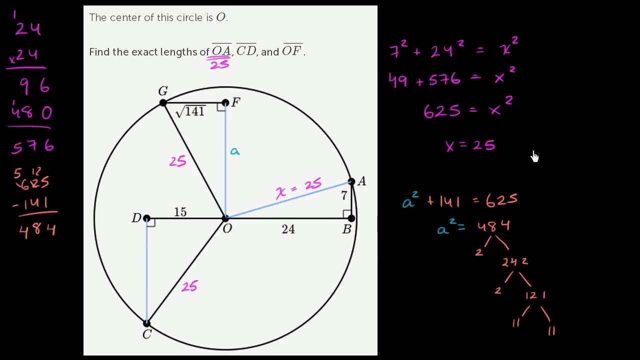 So another way of thinking about it is: this is 2 squared, So 484, all right over here. 44 is equal to 2 squared times 11 squared, or it's the same thing as 2 times 11 squared. 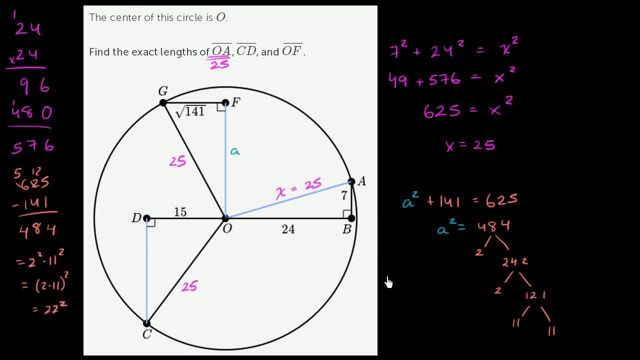 So 484 squared, which is 22 squared. So in this case a is equal to. let me just clean all that up so I have some space to work with. a is equal to 22.. Let me write that down: a is equal to 22.. 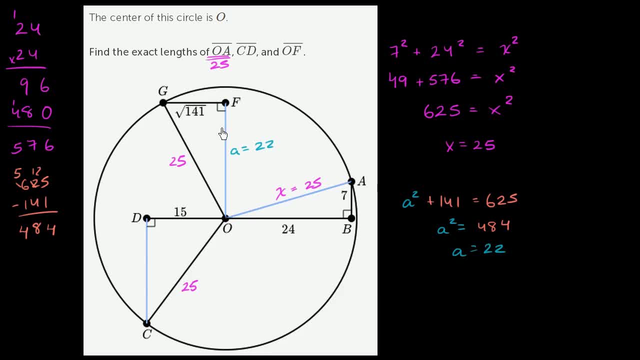 So that's equal to 22, right here, And that's the length of segment OF. So this is 22.. And then finally, CD. Once again, we just apply the Pythagorean theorem. Let's just call this. I've already used a. 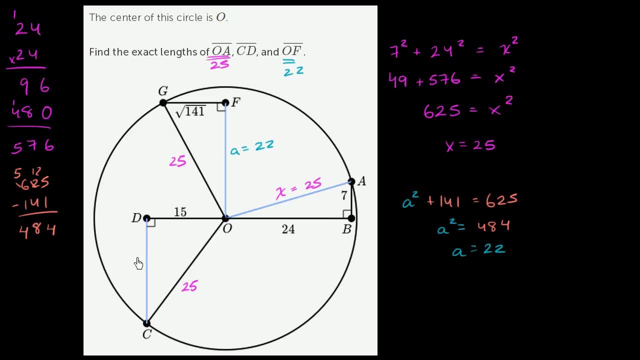 I've already used x, I don't know. I'll call this b. I'll call this length b. So we see that b squared plus 15 squared, which is the same thing as 225, 15 squared is 225,.